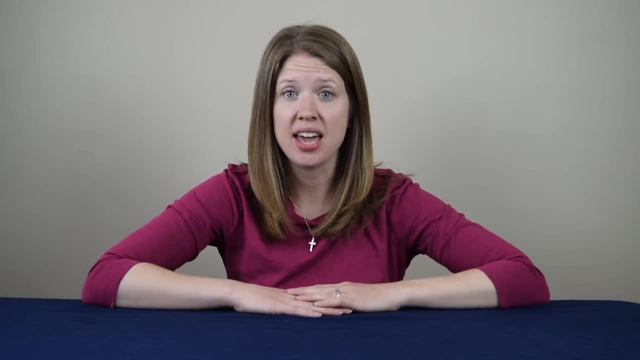 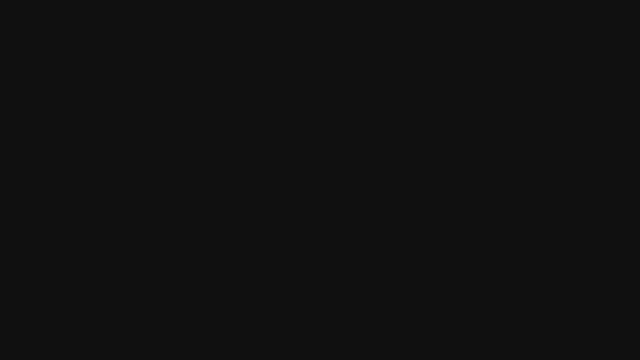 Hey everyone, it's Danielle from Cool Science Experiments Headquarters, and today I'm going to show you a simple experiment and we're going to learn how different types of materials conduct heat. Are you ready? Let's get started To begin, you're going to take a small glass bowl and inside you're going to place three. 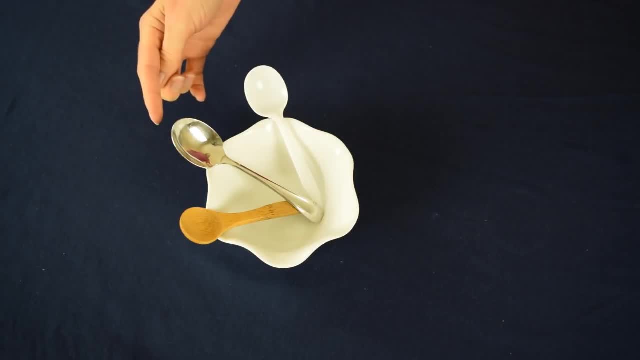 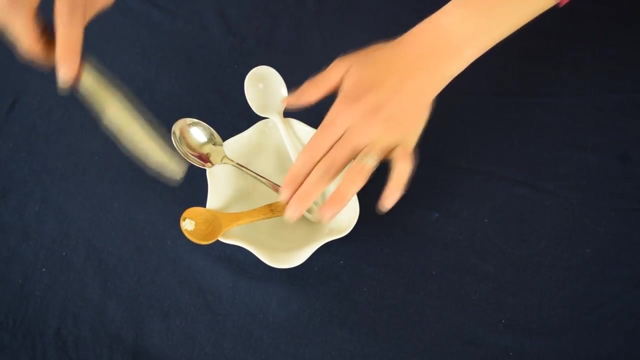 spoons- One spoon that's made of wood, one spoon made of metal and one spoon made of plastic. Then you're going to take a small pat of butter and you're going to place it on the top of each of the spoons. 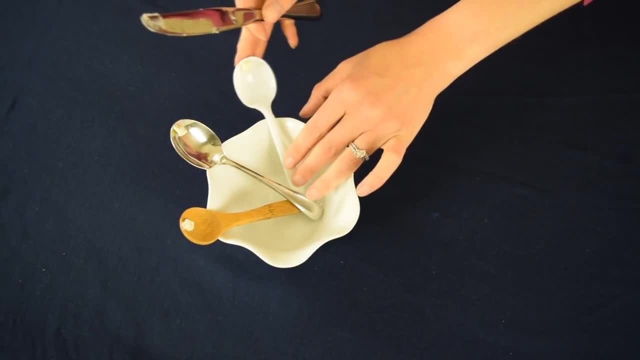 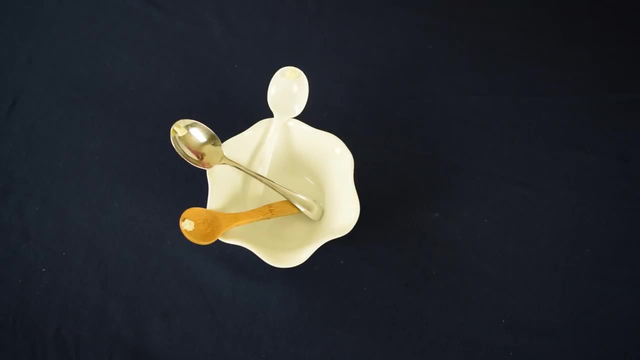 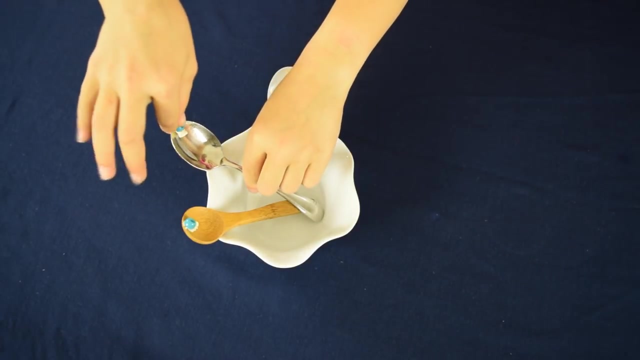 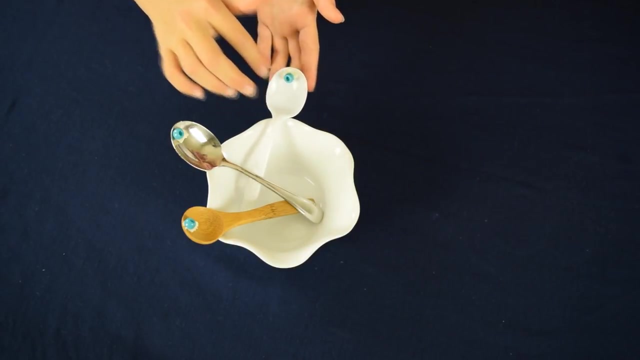 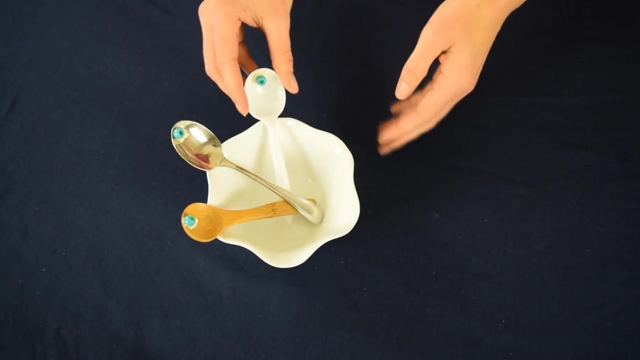 Once you have the butter on the spoons, you're going to put a bead in the butter on each of the spoons as well. Then, after you have the beads and the butter on the spoons, you 're going to straighten out the spoons so they're all laying evenly. 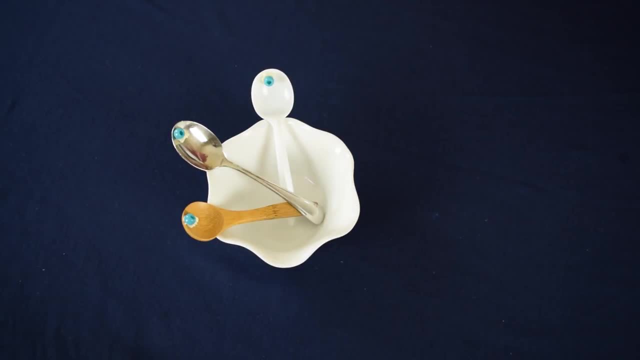 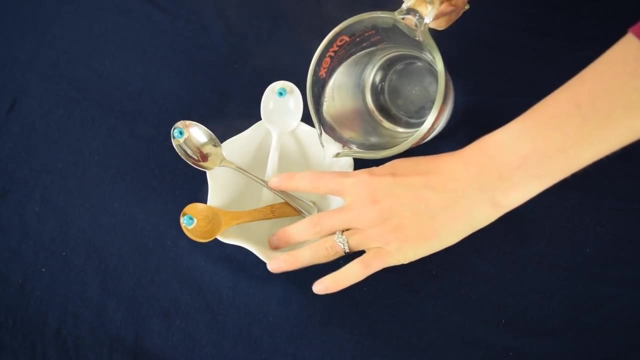 Now it's time to move to the next step. For the next step, you're going to take some hot and just boiling water and you're going to slowly pour it into the bowl. You want to make sure that the spoons do not fall into the water. 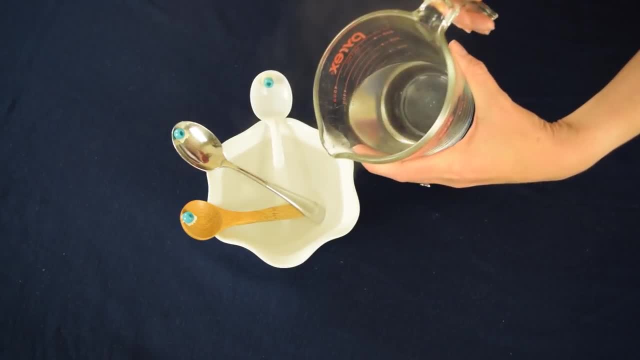 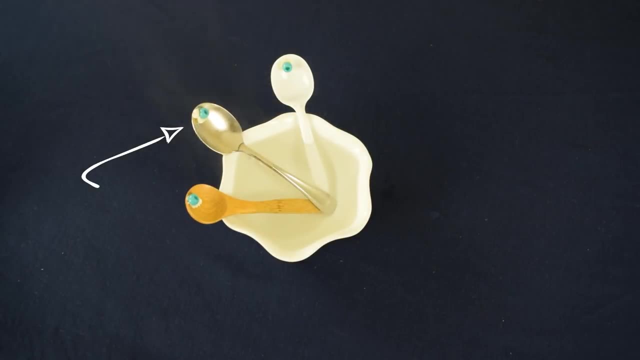 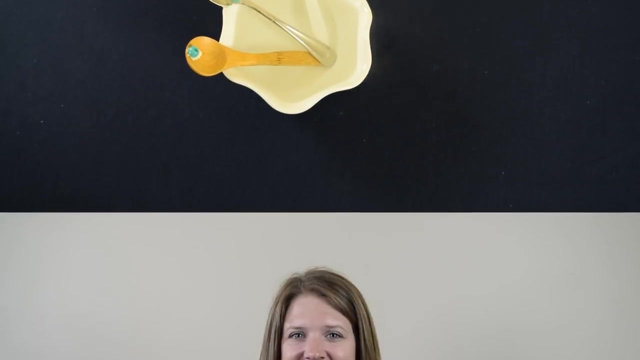 Once you have the water in the bowl. we're going to wait and we're going to watch to see what happens. Can you tell me why did the bead move down the spoon? that was made out of metal, but it stayed at the top of the spoon. 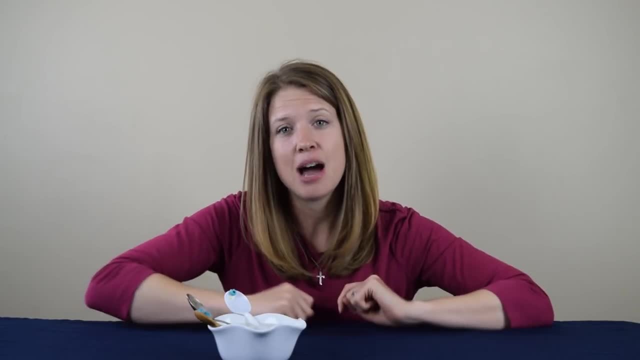 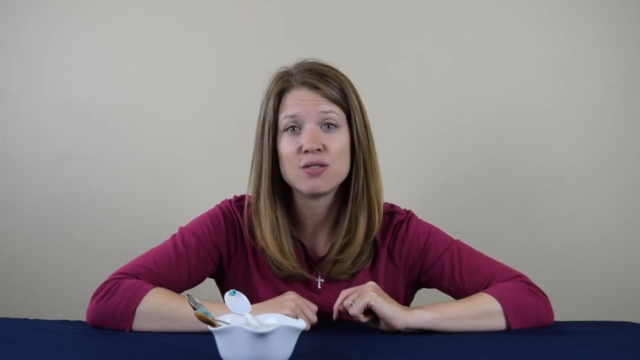 Why did the spoon move down? the spoon that was made out of wood and plastic. Leave a comment below to submit your guess and then visit CoolScienceExperimentsHeadquarterscom to find out the answer. You'll be able to print out instructions for this experiment.